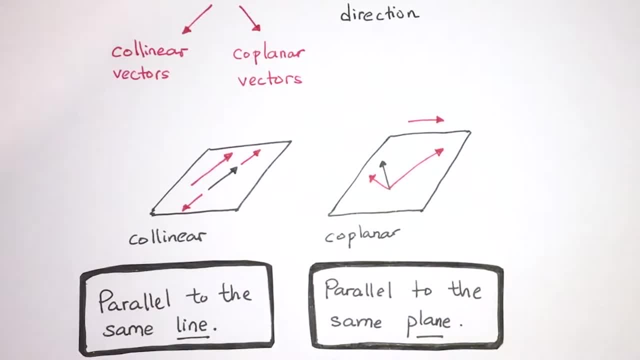 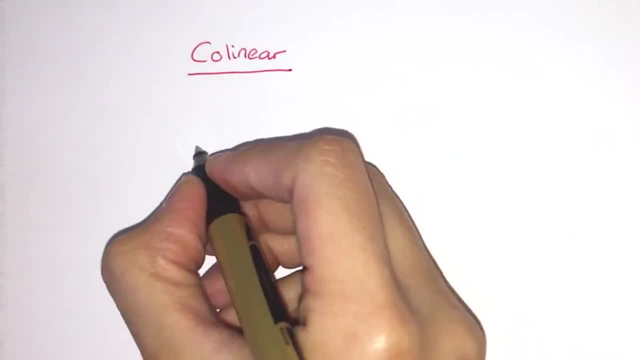 And you can also see that by default all collinear vectors are also coplanar. Adding vectors that are collinear is relatively simple. You would have met that already in GCSE physics. So first let's look at the vector quantity. 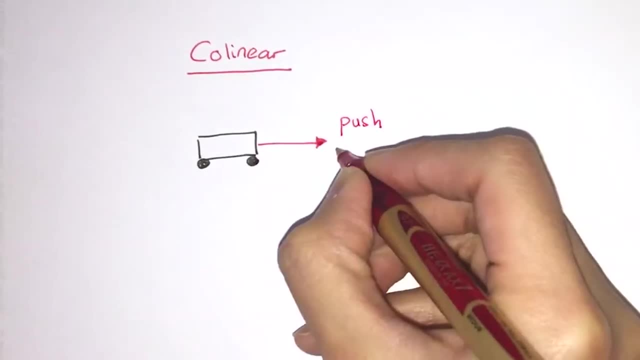 So, for example, if I have a vector that is parallel to the same line, for example, if we have a car being pushed in one direction with a force of 10,000 newtons and the friction acting on the wheels is 3,000 newtons, 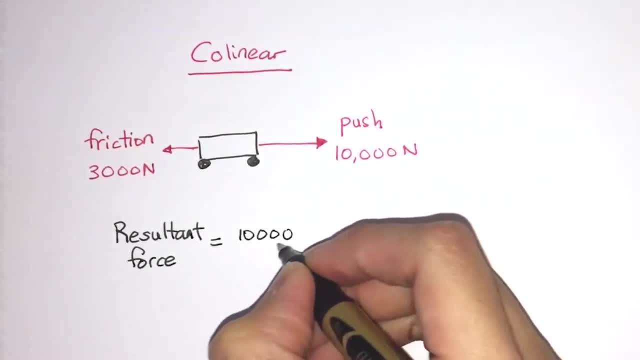 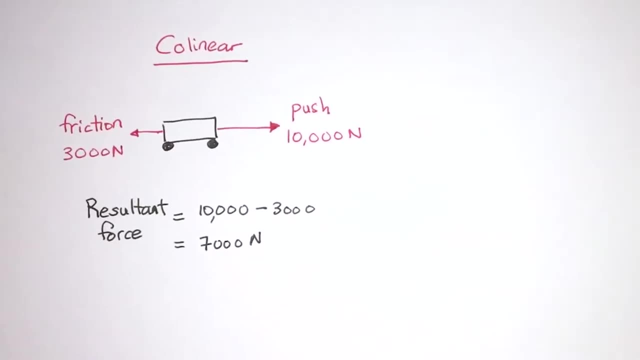 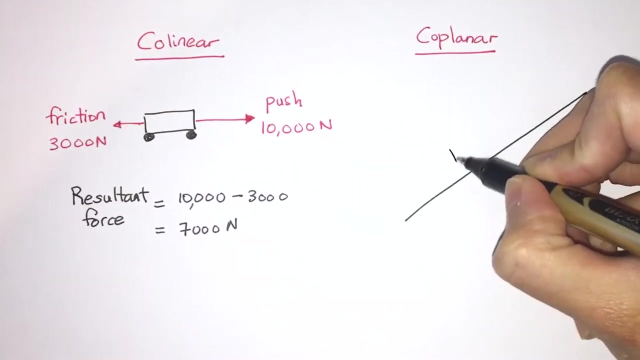 then the resultant force is simply 10,000 minus 3,000, and you get 7,000 newtons as a resultant force. And this is for forces that are collinear. But when you have coplanar forces that are not collinear, it complicates things a little bit. 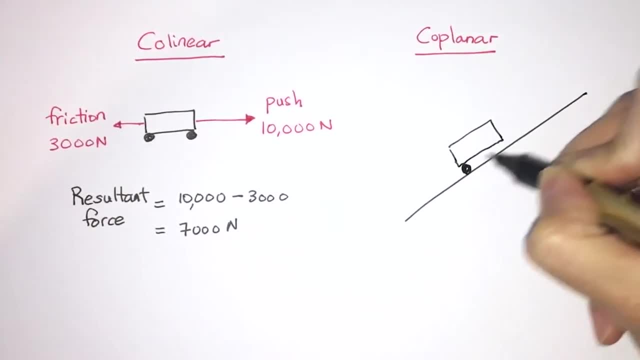 So here's a coplanar. Here's a coplanar situation where you have a car being pushed uphill and you have weight acting downwards towards the center of the earth. You have the push, you have the friction, you have the normal reaction force between the wheels and the slope. 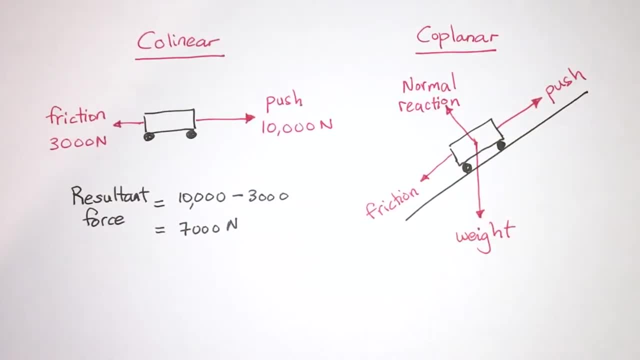 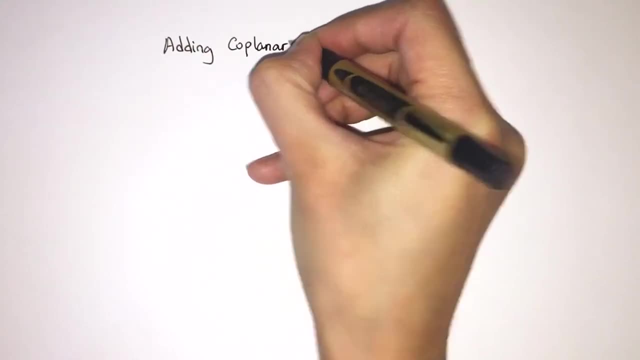 You have all of these forces acting on it. So even if you don't have forces that are acting parallel to each other, you still need to know how to add them together. I'm going to show you how you can add coplanar vectors together. 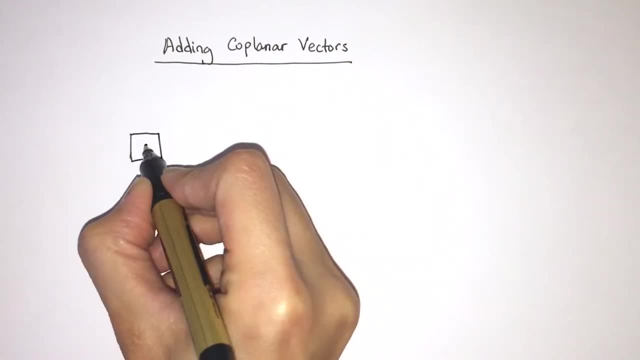 Here we have an object and there are two forces acting on it. One is horizontal- 4 newtons- and the other one is vertical, and that's 3 newtons. We're going to use the method known as the head-to-tail method. 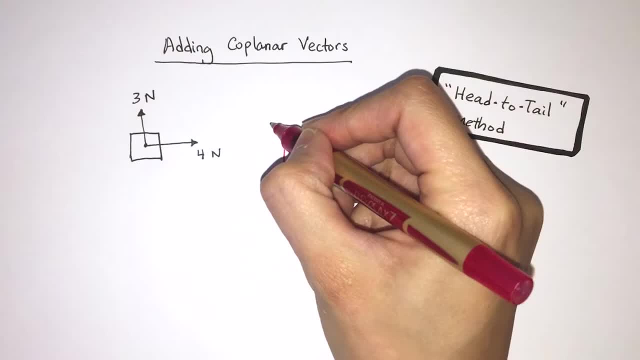 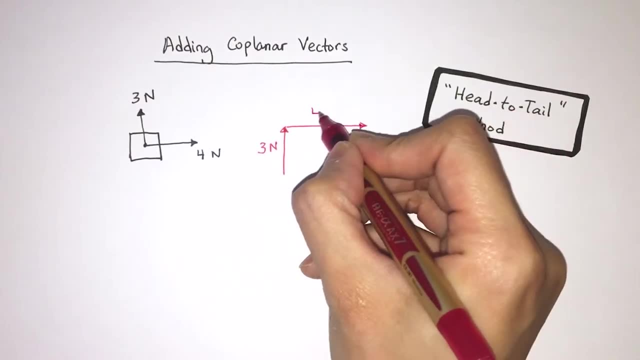 I'm going to draw the 3 newtons force. first, Take the end of the 4 newton arrow and attach it to the head of the 3 newton arrow. Then I'm going to complete this triangle with a dotted line. 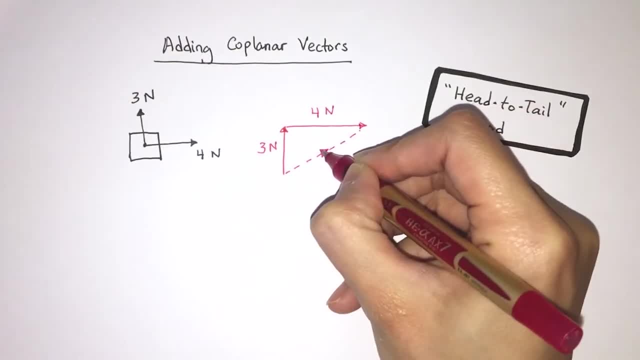 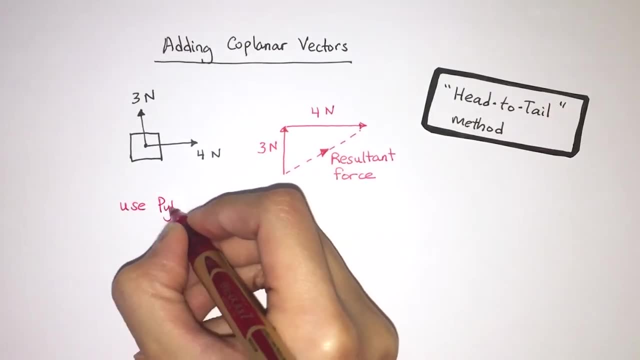 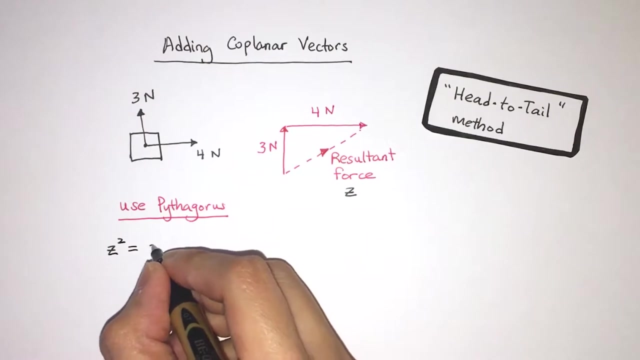 and the dotted line is my resultant force of these two forces, Then I'm going to simply use Pythagoras. So Pythagoras' theorem says that z squared is equal to x squared plus y squared. So I'm just going to square root all of those to get z. 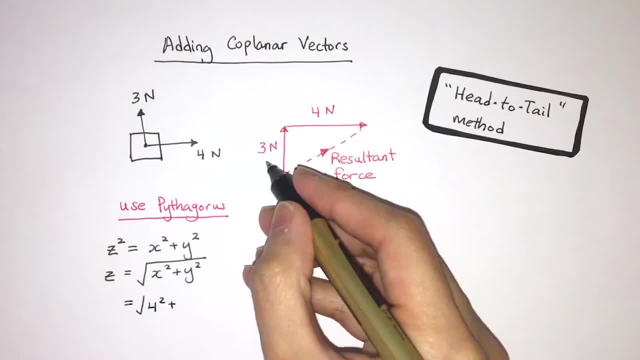 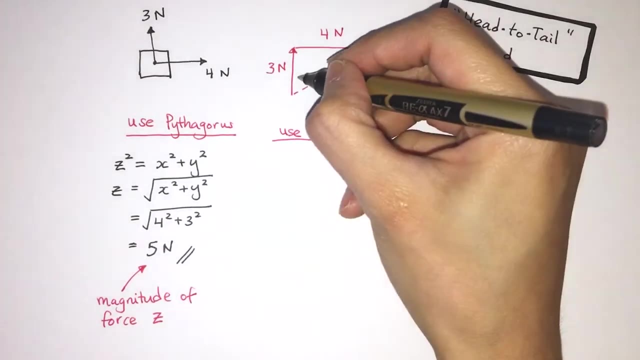 and that's square root of 4 squared plus 3 squared, and that gives me 5 newtons. 5 newtons is the resultant force. But I can't just stop there, because a vector also has a direction. So I'm going to use trigonometry to figure out the angle theta. 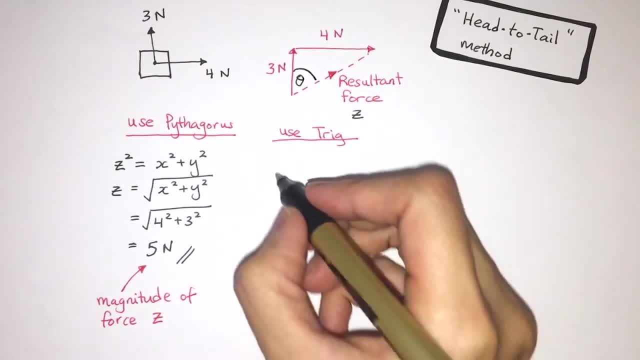 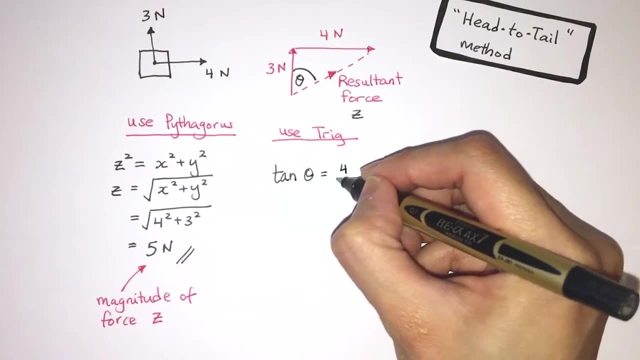 and theta is representing the direction of my resultant force. So tan theta is equal to the opposites divided by the adjacents, and in this case that is 4 divided by 3.. That gives me an angle of 53.1 degrees. 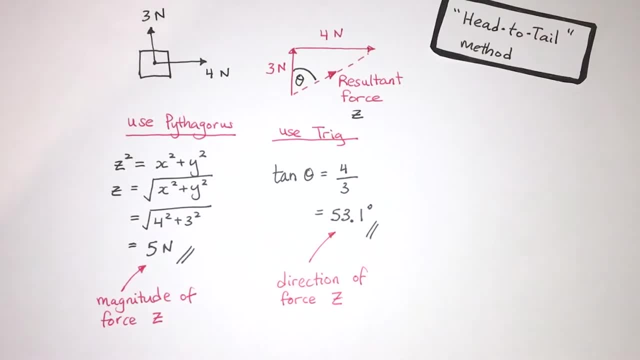 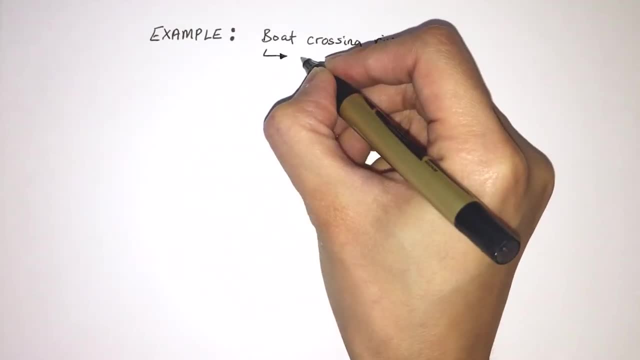 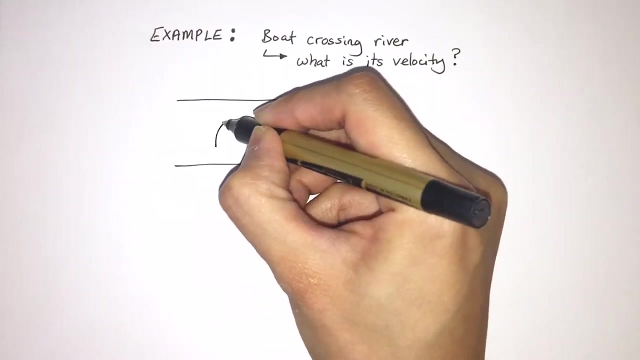 That is the direction of my resultant force. Let's look at an example where we have to figure out the resultant force of coplanar forces. A rower is trying to get from one side of the river to the other side of the river by rowing his boat. 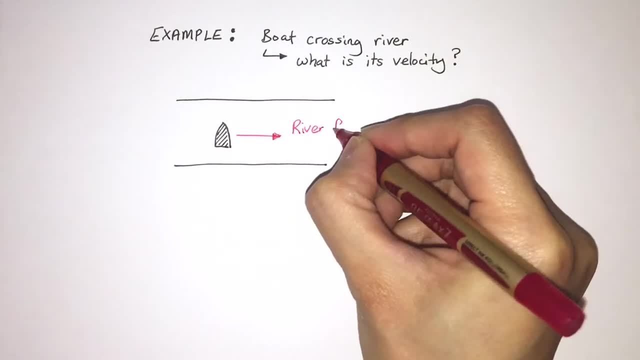 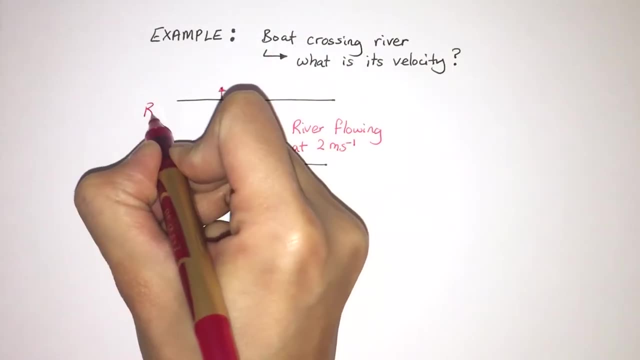 But there's a water current flowing down the river at 2 meters per second. The rower tries his best to row directly across the river vertically at 1 meter per second, But since there are two different velocities, trying to pull the boat in different directions. 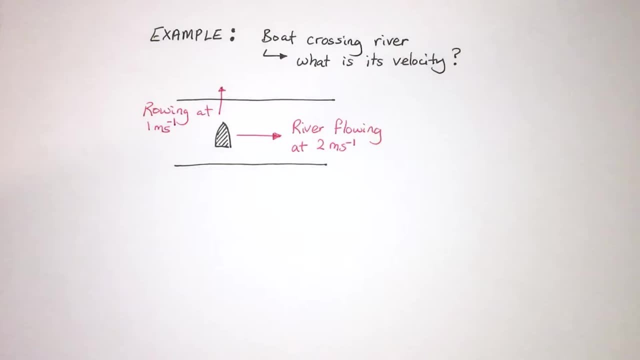 the water trying to pull it to the right, the rower trying to row forward. the boat will actually travel diagonally. We want to figure out the boat's resultant velocity And again we use the head-to-tail method. I redraw this diagram again. 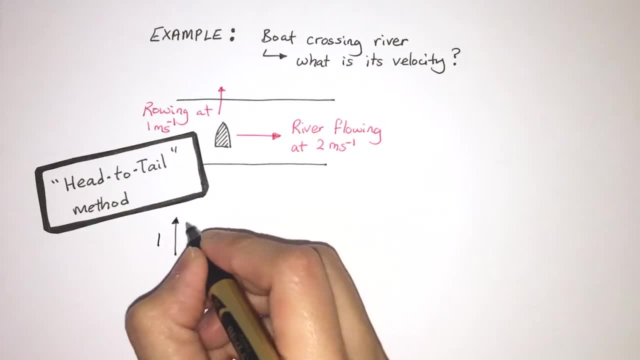 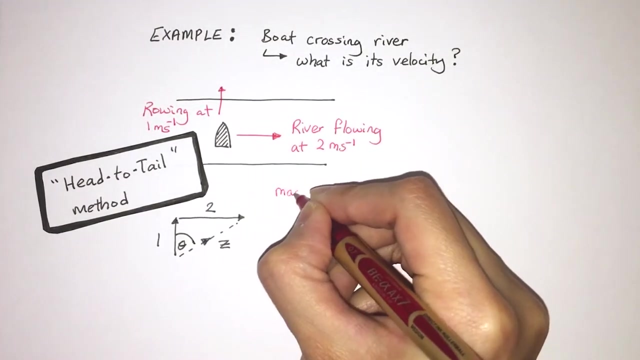 starting with the vertical arrow, and that's 1 meter per second, And my horizontal arrow is 2 meters per second. The dotted line is showing the resultant velocity And angle. theta is the direction of this new velocity. To find a magnitude again, I use Pythagoras. 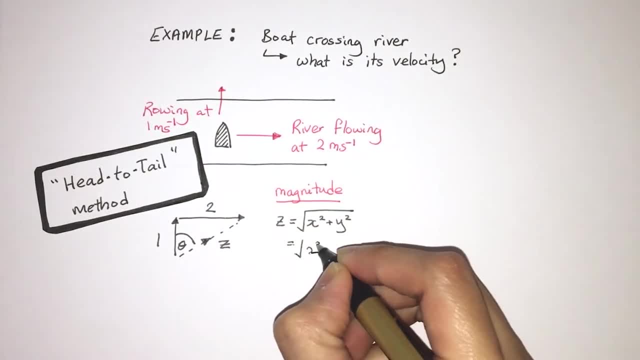 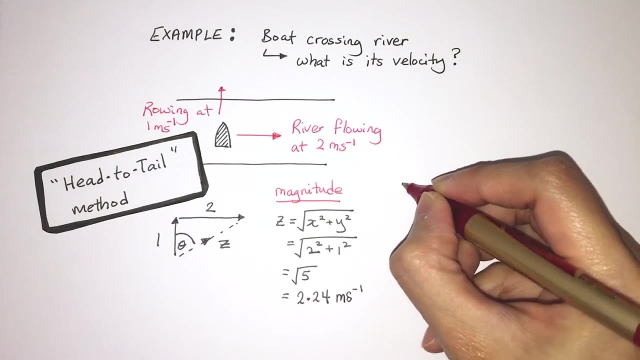 And that is just 2 squared plus 1 squared, and then all of this square roots, Square roots of 2 squared plus 1 squared, And that gives me 2.24 meters per second. And to find a direction, I do 10 theta. 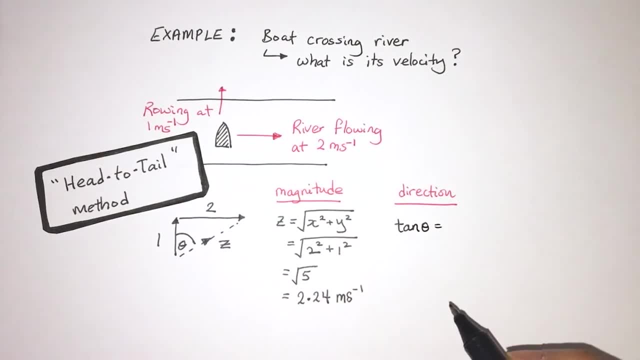 is equal to the opposite over adjacent, and here it's 2 divided by 1.. That gives me an angle of 63.4 degrees. In other words, the boat is going to travel at 2.24 meters per second at an angle of 63.4 degrees from the north.